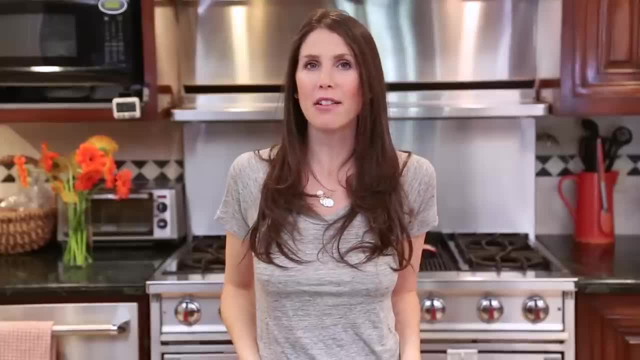 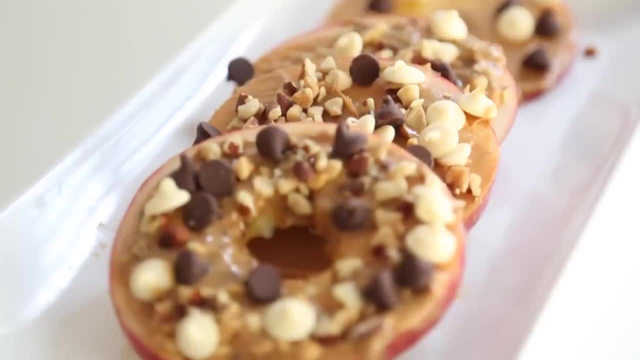 Hey guys. So if you're like my family, there was a lot of indulgence over the holidays, but I've definitely found with kids it's super hard to go cold turkey. So today I'm going to show you guys three healthy alternatives to start your new year off right. I'm Meg. 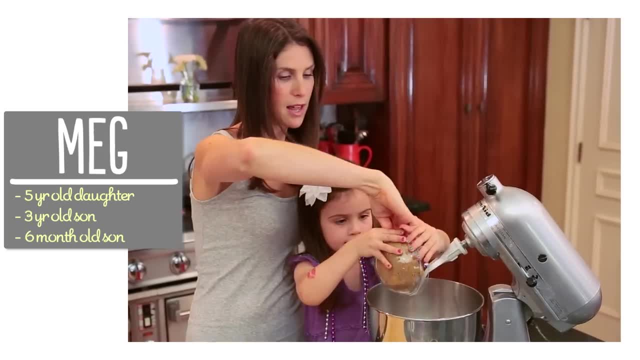 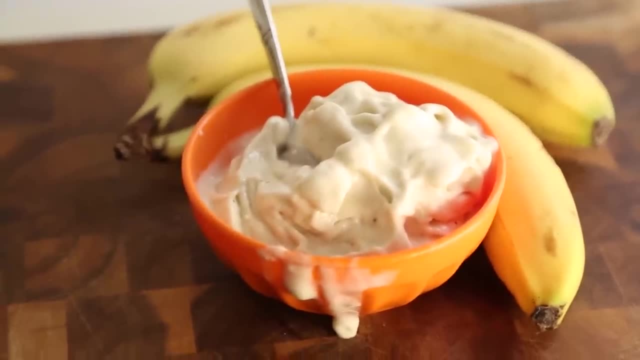 and I'm passionate about finding ways to make life with kids easier in the kitchen. All right, so first up, we have one ingredient: banana ice cream. All you're going to need is some bananas. Now what I like to do is use super ripe bananas. I cut them up into like one to two. 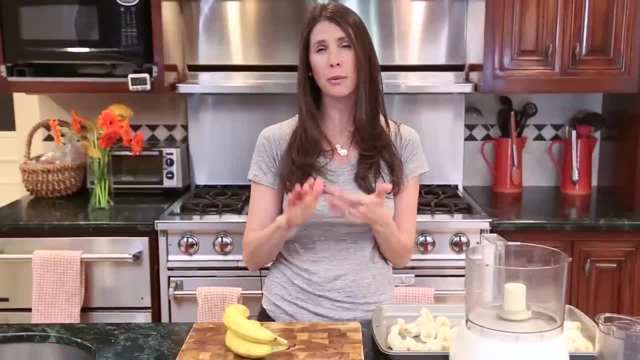 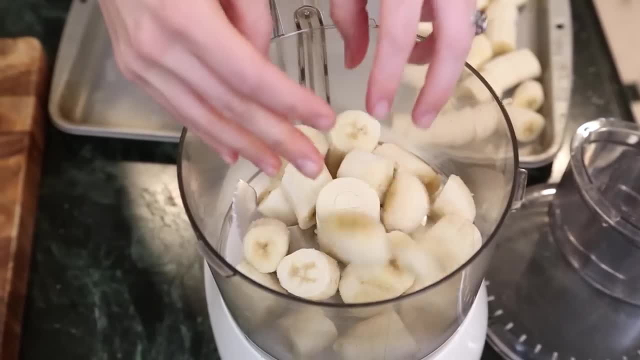 inch sections and freeze them for at least two hours, up to overnight- I really feel like overnight is a lot better- And then what you're going to use is your food processor or a really high-powered blender, and all you're going to do is puree them. All right. so occasionally we'll get stuck. 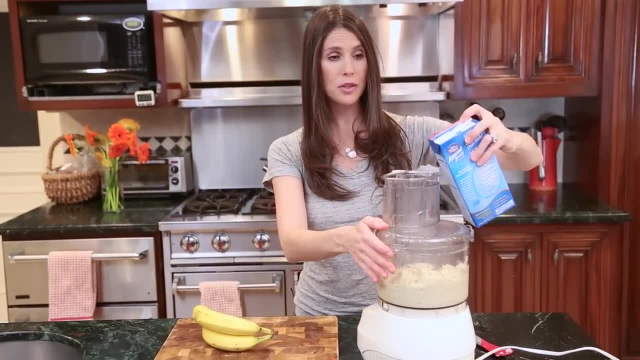 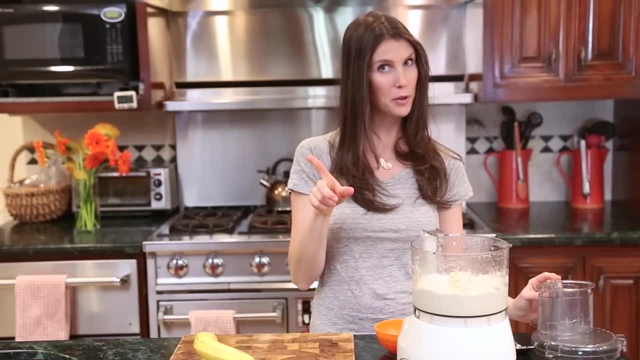 which you can see today. So I'm going to show you guys how you can just add a little splash of milk to help things get going Now. I promised you guys it was one ingredient and then I added the milk, but that was off. I'm going to take them to the blender now And then I'm going to 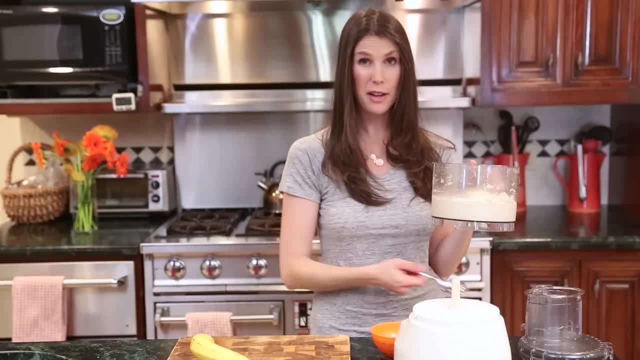 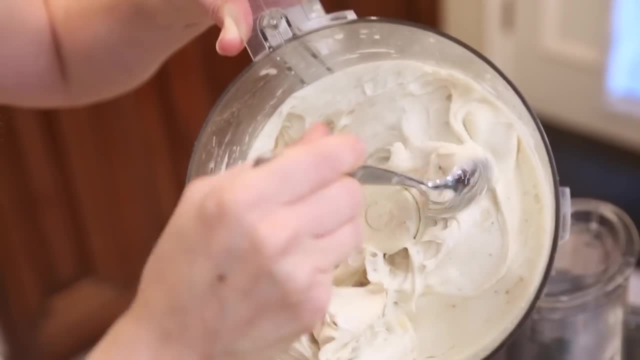 The other thing that you guys can do is actually change the flavor, so you can add a little bit of peanut butter when it's pureeing, or you can add some frozen strawberries and then you have a totally different flavor to mix it up. You can see that the texture is just really great. It tastes just like soft serve. 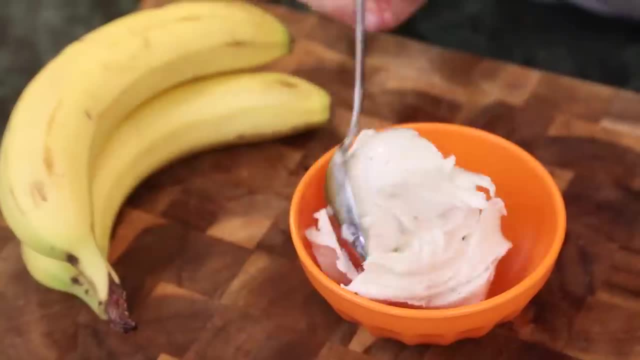 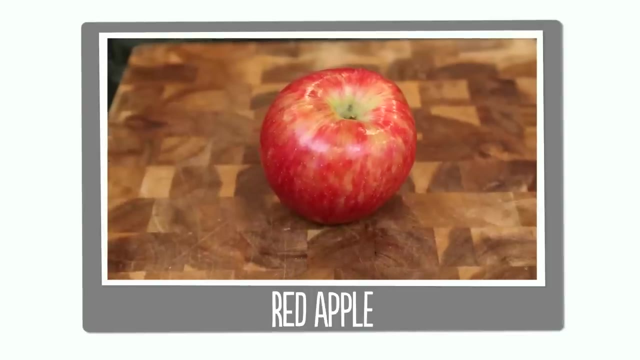 ice cream and you can stick it in your freezer if you want it to be hard serve. So banana ice cream. there really couldn't be anything simpler. Next we have apple cookies, and here's what you're gonna need: A red apple nut butter. 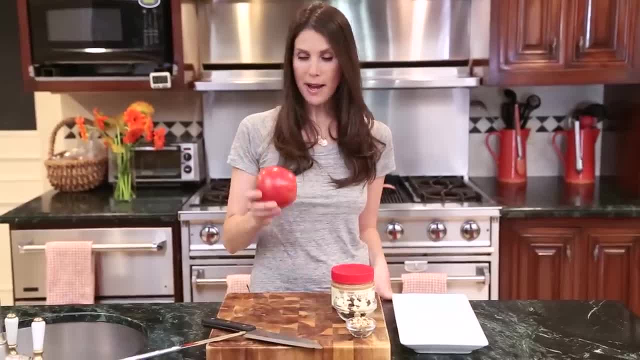 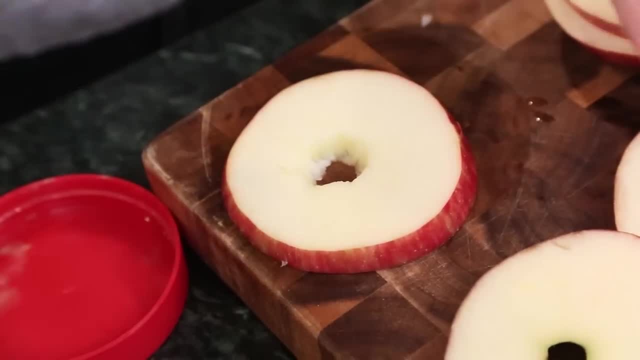 nuts and chocolate chips. Alright, so I've already washed my apple. the next thing I'm gonna do is slice it into rings, and then I'm gonna take the core out after, just by cutting around with my knife. An apple core would also work very well, but 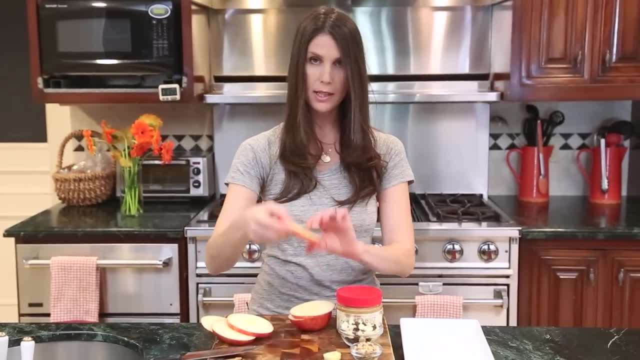 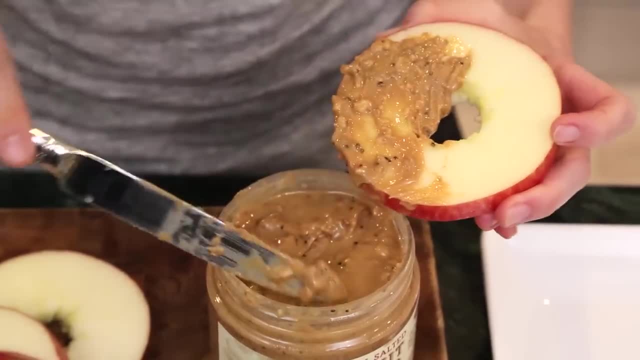 I'm just not that fancy and I do not have one. So I've got my apple slice all ready to go and next I'm gonna use my nut butter. Now you can use almond butter, plain peanut butter. I actually just found this one that's a peanut butter. 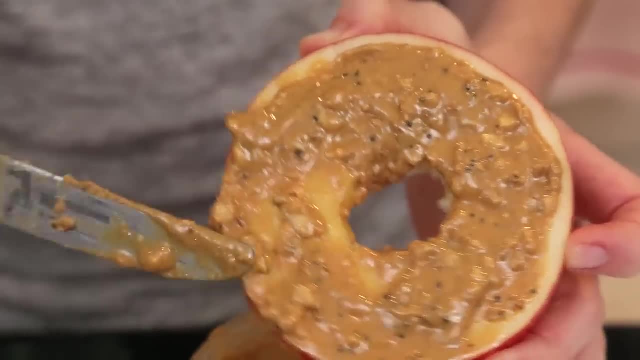 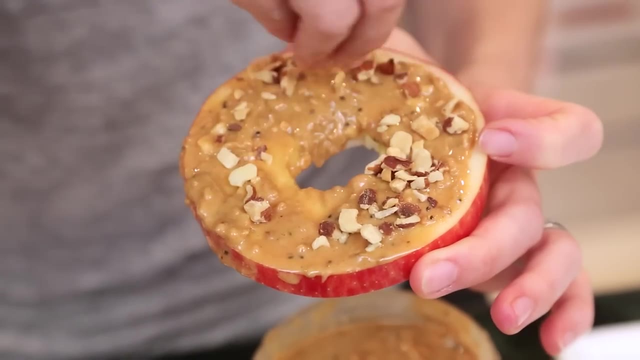 and it has flax and chia seeds in it, so you know extra nutritional benefits. I thought why not? And after my butter is on there, I'm just gonna sprinkle my topping. So today I've got some roasted almonds that are nice and chopped up.